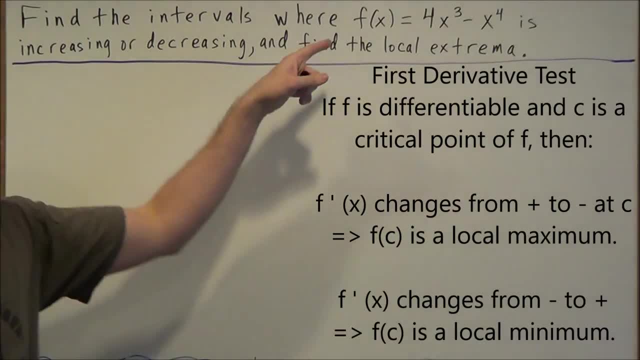 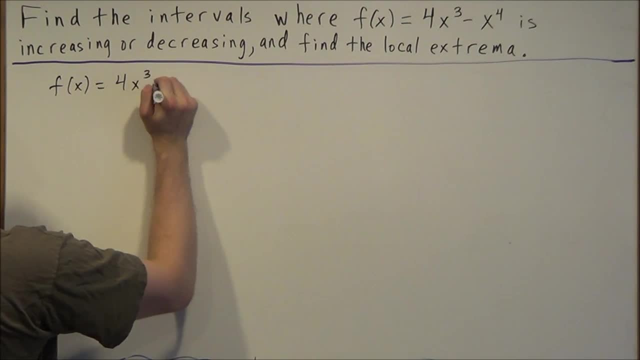 So to answer this problem, we're going to use the first derivative test. We're starting off with f of x equals 4x to the third minus x to the fourth, and the first thing we want to do is find the derivative. So we'll have f prime of x equals and using power rule. 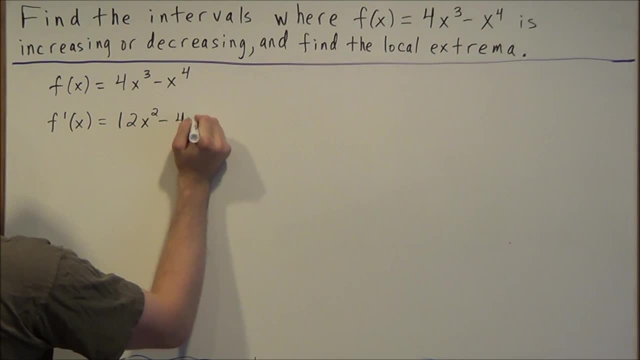 the derivative is 12x squared minus 4x to the third. So at this stage here we're going to find the critical points. so we're going to factor the derivative and set it equal to zero. We'll have f prime of x equals f prime of x. 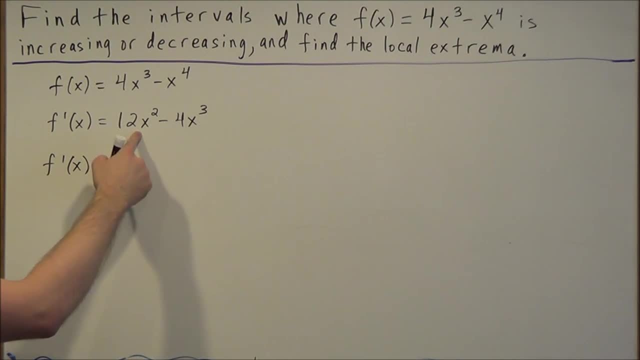 prime of x equals, and if we find the greatest common factor- in this case it's 4x squared and left over in parentheses, we'll have 3 minus x. So we set this derivative here equal to 0 to find the critical points. 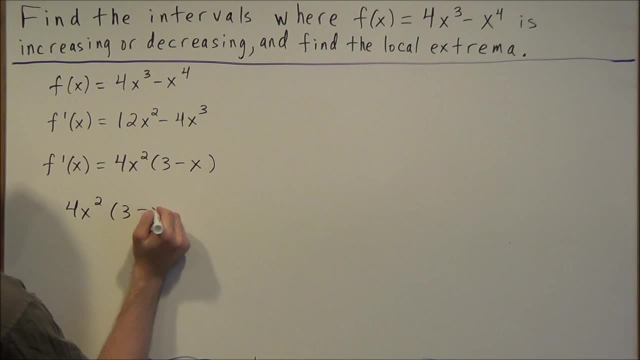 And we have 4x squared times: 3 minus x is equal to 0.. Now this first factor here, 4x squared- is equal to 0 when x equals 0.. And the second factor, 3 minus x, is equal to 0 when x is equal to 3.. 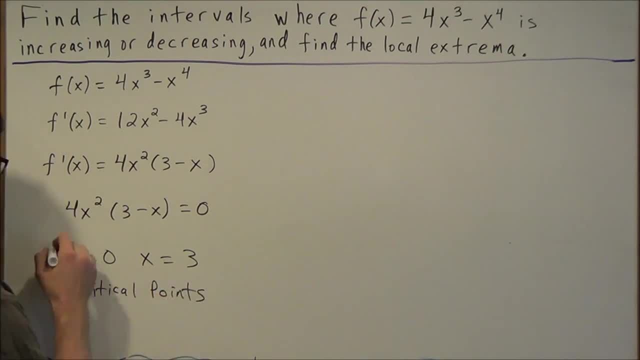 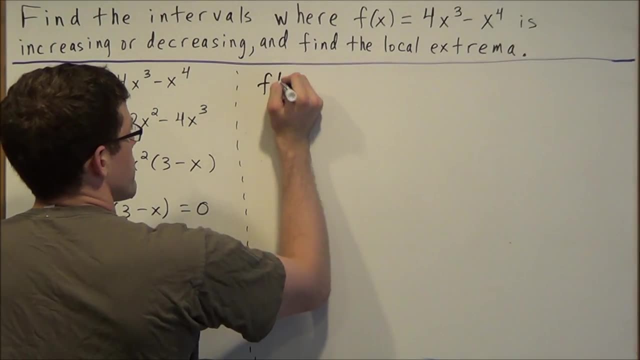 So these values here represent our critical points. So for the next stage of this problem we're going to make a sign chart for the first derivative- So we have f prime- And for the critical points we found here, we're going to mark this on the number line. 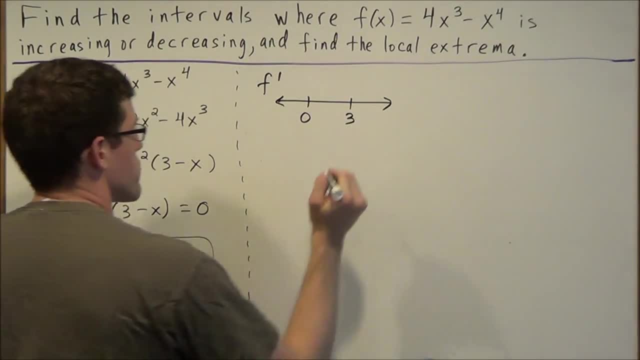 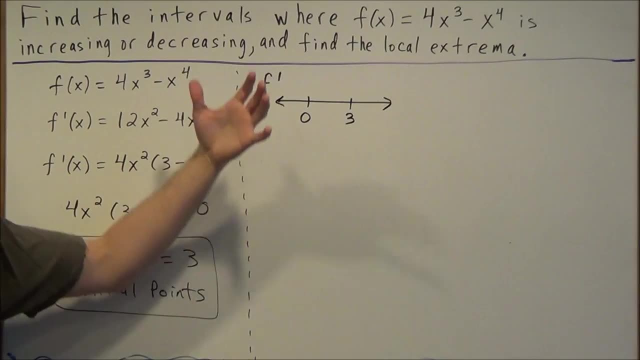 So we're going to make a mark here and at zero and a mark at three. And now notice here: this creates three intervals and for this stage of the problem, with enough practice, if you're skilled with mental math, you could do this part in your head. However, when you're first starting out with this, I would recommend writing out the 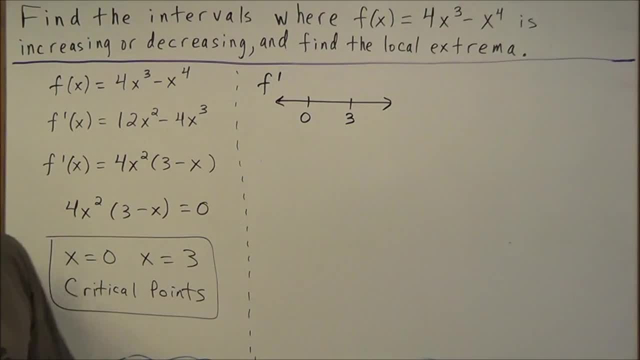 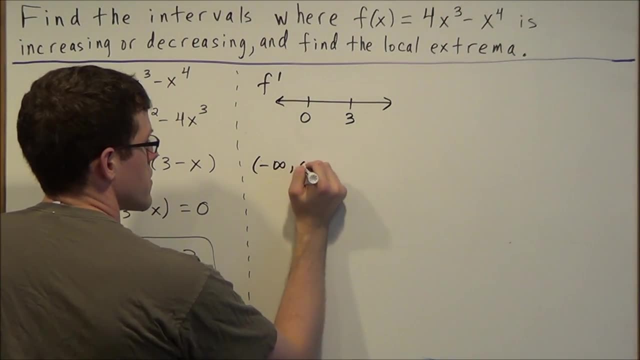 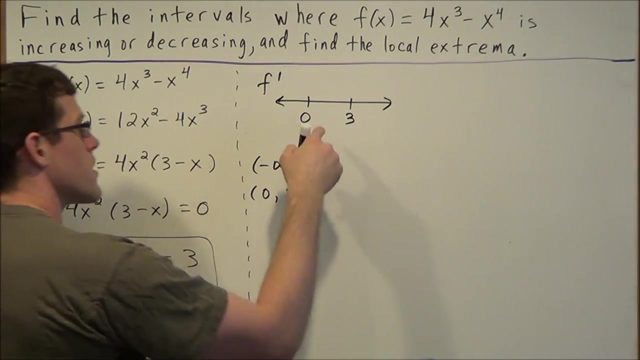 steps. that way your answer is more accurate and you get the full credit. So the first interval for this number line goes from negative infinity to zero. The second interval goes from zero to three and the last interval goes from three to infinity. And what we want to do is we're going to pick a. 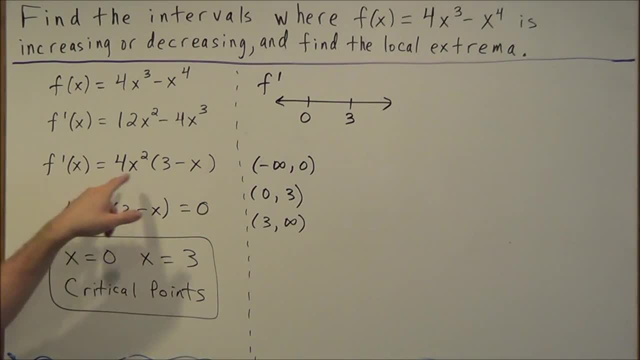 number in each of these intervals, plug them into the first derivative and record the sign. All we care about is the sign, we don't care about the value. So for this first interval, here the interval goes from negative infinity to zero. The second interval goes from zero to three. 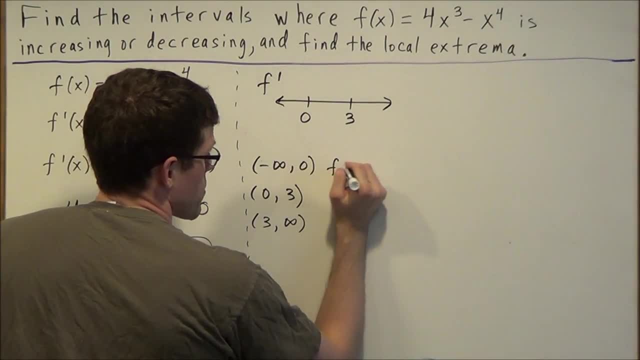 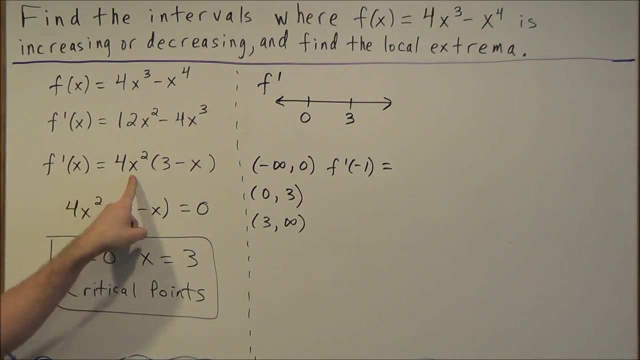 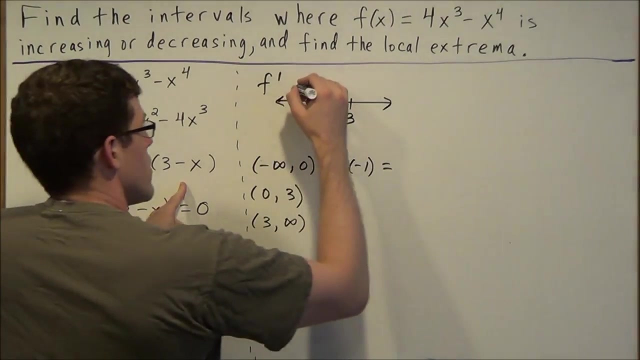 The easiest number we could pick out is negative one. We're going to plug negative one into the first derivative and if we were doing this in our head we would say: four times negative, one squared is positive, Three minus negative, one is positive and a positive times a positive is positive. So 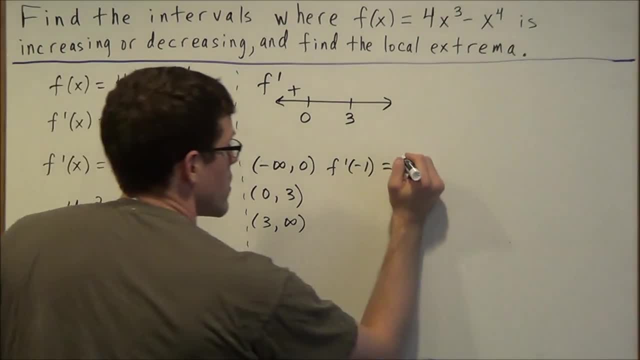 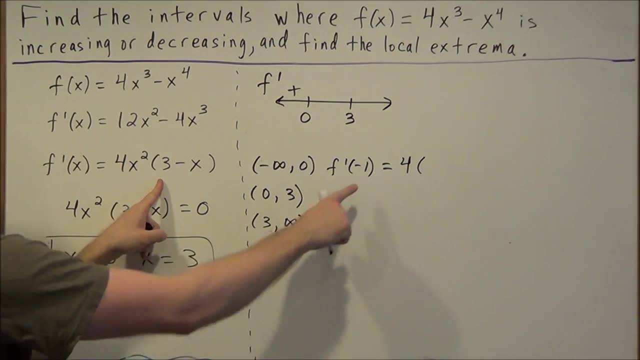 that would be like the fast way of doing this. but if we write this out, we have four times negative one squared, which is positive one, and we have times three minus one squared, which is positive. three minus negative one gives us four, and this equals positive 16 and we record the sign in that. 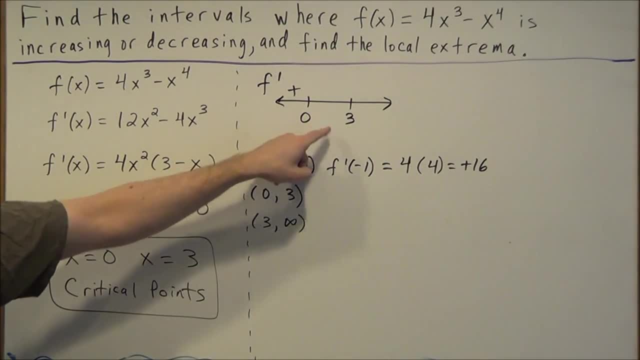 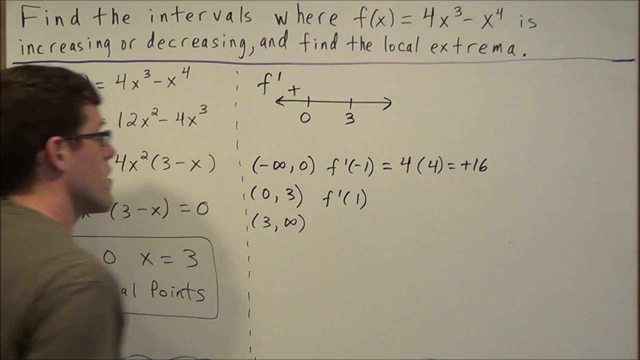 interval. here And now we repeat this. so we have to pick a number between zero and three. The easiest number we could plug in is one, and we're plugging this into the first derivative. And just know, you could plug it into either one, but for most problems if you plug it into the factored. 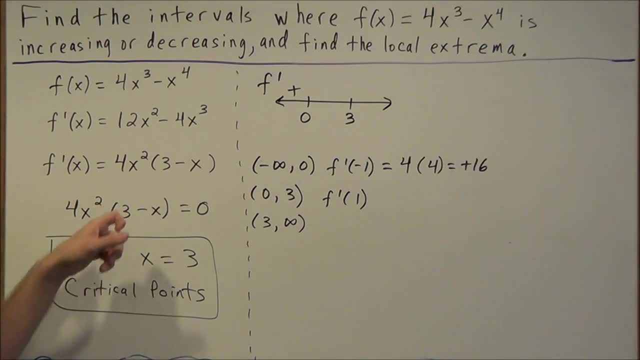 form, you're able to say that concept out loud, like the positive times a positive. So the factored form allows you to do this method in your head when we're working at this part here. So if we plug in one, we could say four times one squared is positive. three minus one is positive. 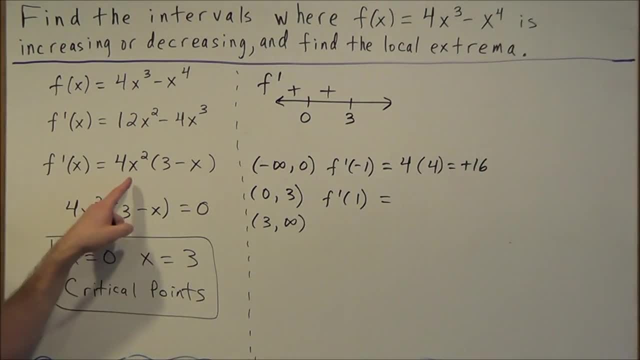 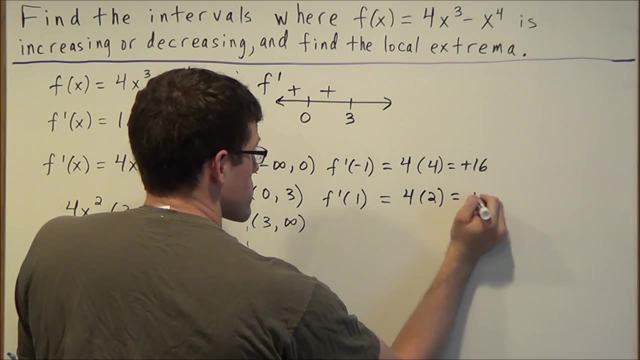 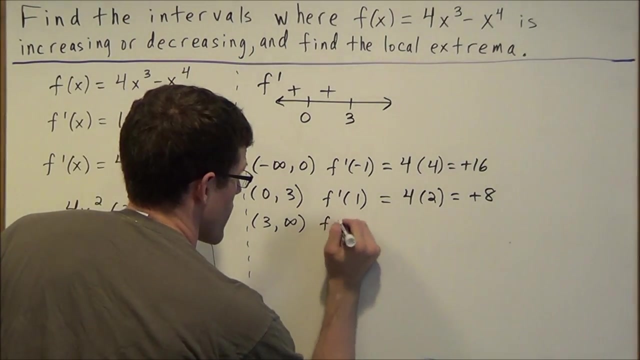 and a positive times. a positive is positive, But if we write it out formally, this is four times one squared, and then three minus one is two and this is equal to positive eight. So we record our positive sign here and now. for the last interval, we could choose four. We'll have f prime of four equals and. 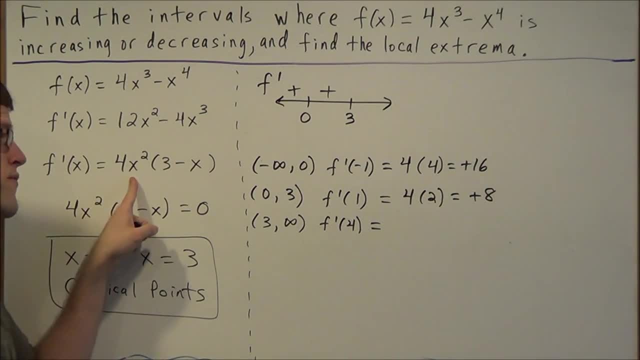 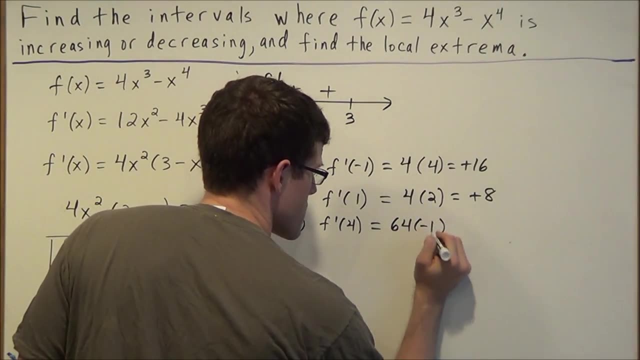 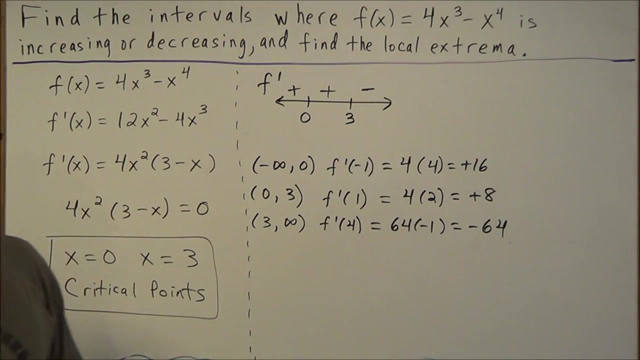 if we plug in, we'll have four times four. squared is four to the third, which is 64 times three minus four is negative one, and this works out to negative 64.. Now just to point out here: the most common mistake with this problem is that students will plug in to the first. 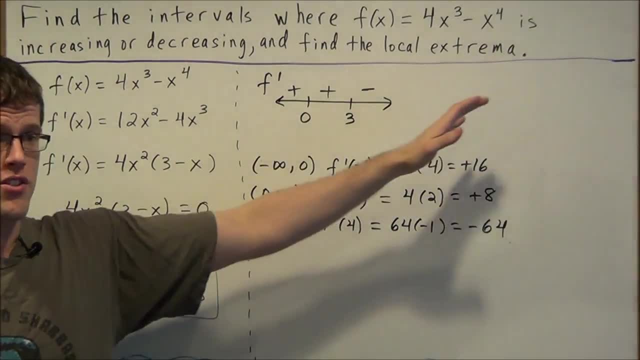 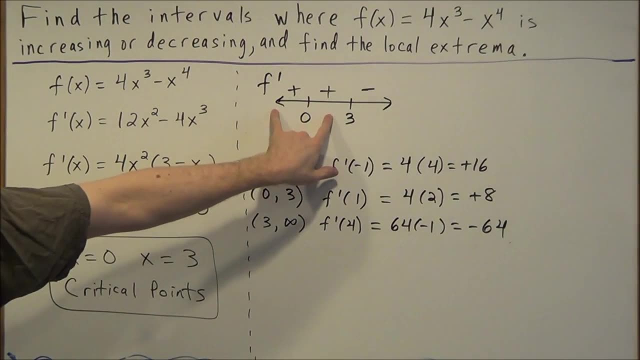 interval. they record the positive and they assume that it changes from one interval to the next. So they find one and they say positive, negative, positive. but in this case here- notice- at zero, there was no sign change, and that's going to be very significant when it comes. 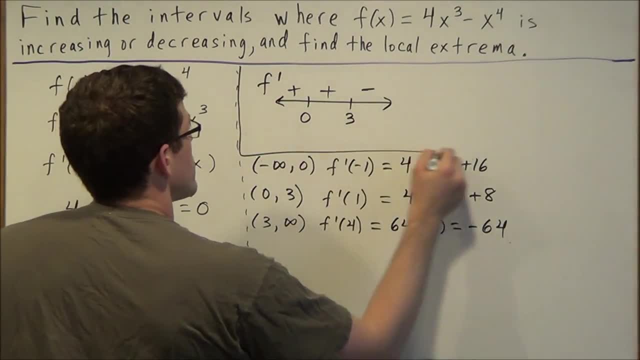 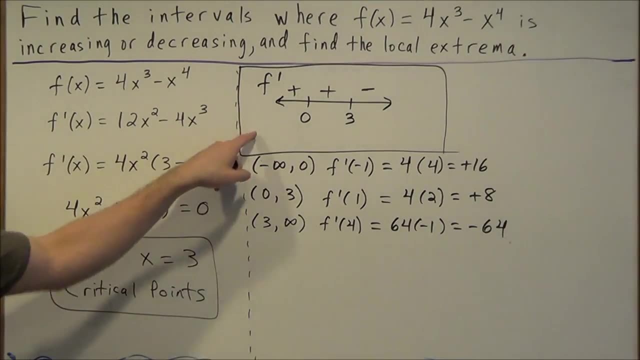 to writing our answer out And just know what we have. here is the most important part of this problem. Once you find the sign chart for f prime like, you're basically ready to go and answer it. So one thing we can look at here is the behavior of f of x. If f prime of x is positive, that means 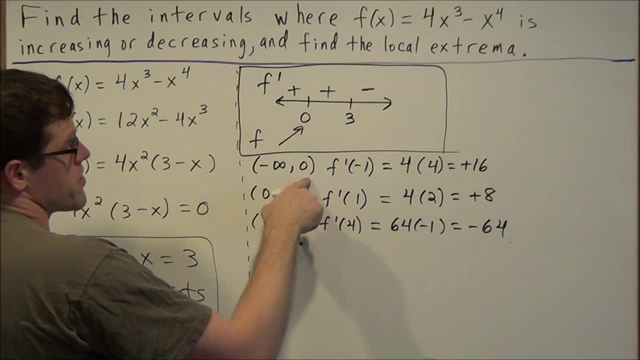 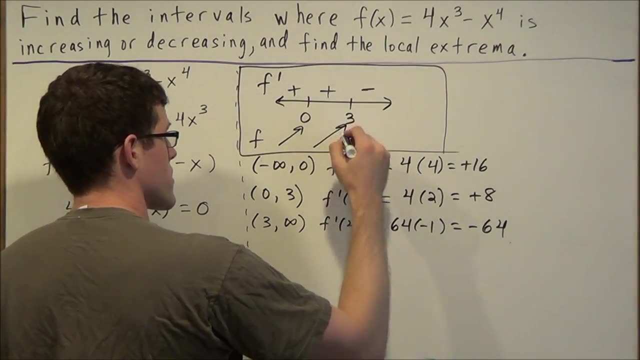 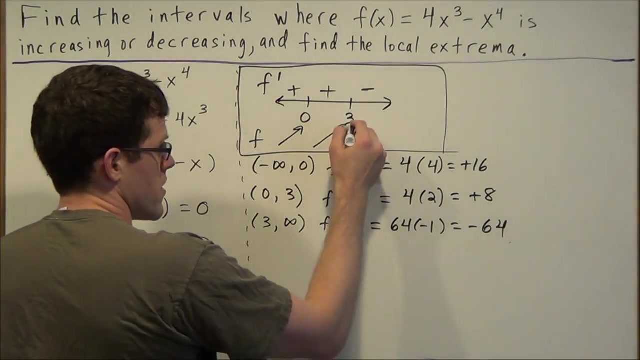 f of x is increasing. So from negative infinity to zero, f is increasing From zero to three, our first derivative is positive, which means that f of x is still increasing, And then from three to infinity, our first derivative is negative, which tells us the behavior of f of x, that 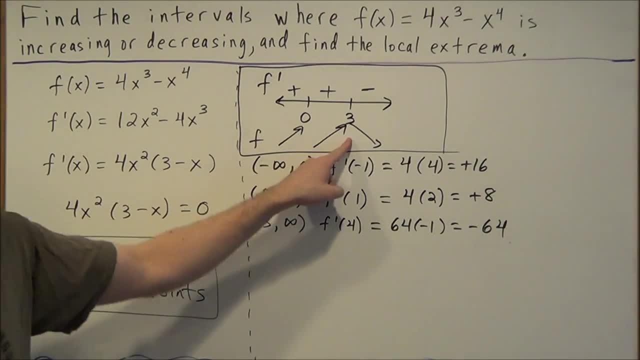 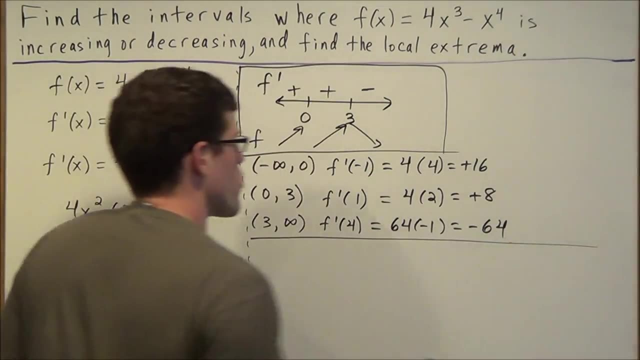 the function is decreasing. So notice here at three we're creating a local maximum because the function is going up and then down here. But to write this out, we could say that f is increasing on the intervals from negative infinity to zero and from zero to three. 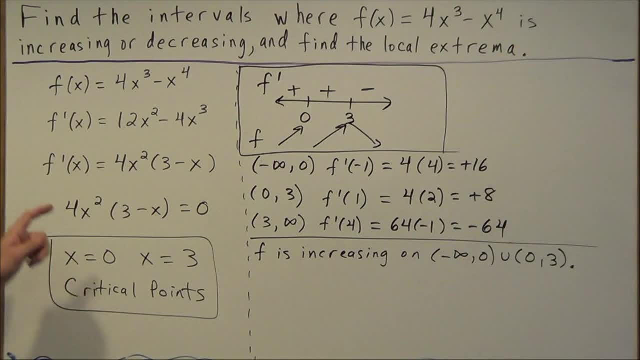 Now it's important to note here that we do not include zero, because the derivative evaluated at zero equals zero. So if your first derivative equals zero, that means at that location the function is neither increasing nor decreasing. So for the next part here, where is the? 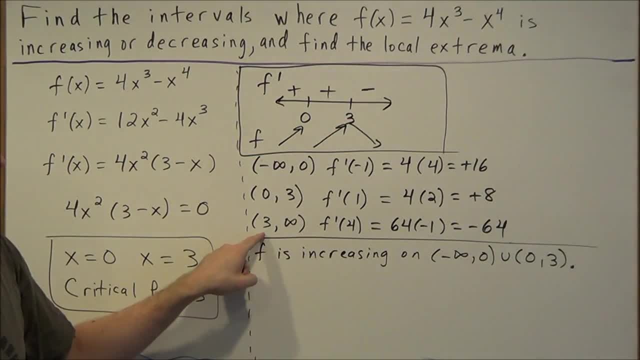 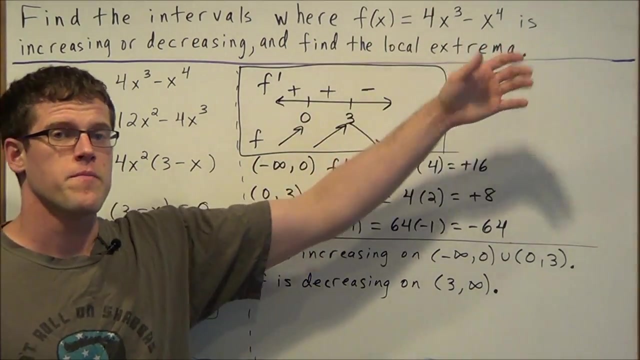 function decreasing. it's decreasing on this last interval, from 3 to infinity, because our first derivative is negative, And if our first derivative is negative, that tells us our function is decreasing. So for the last part of this problem, we're looking for the local extrema. Now 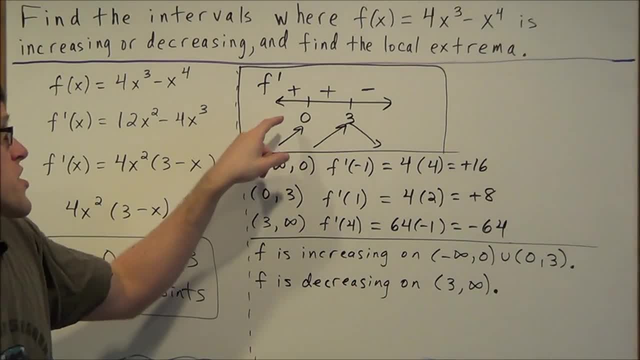 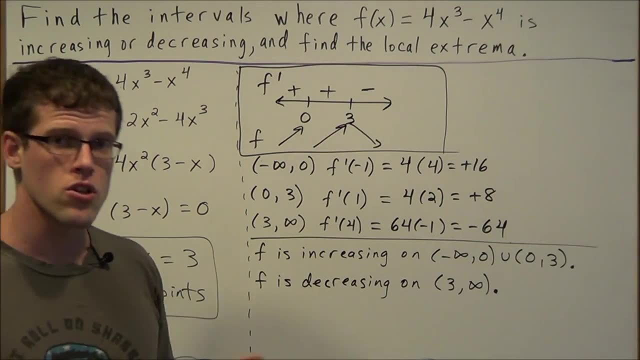 in order for the function to have a local minimum, we would need a sign change from negative to positive. And notice: the first derivative does not change signs from negative to positive, so f does not have a local minimum. In order to have a local maximum, we need the first derivative to change signs. 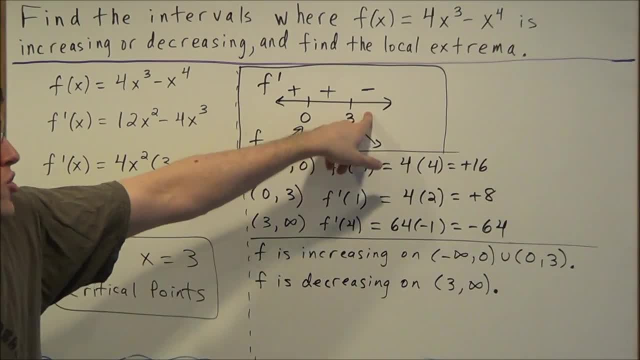 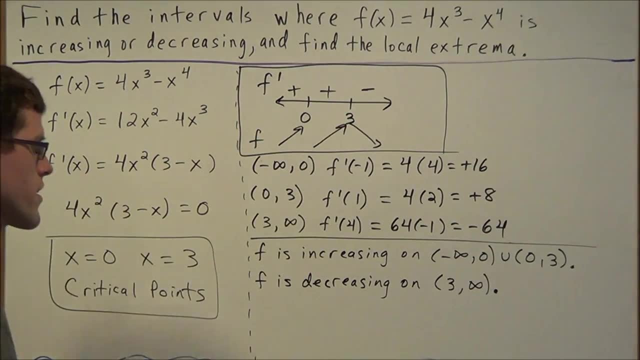 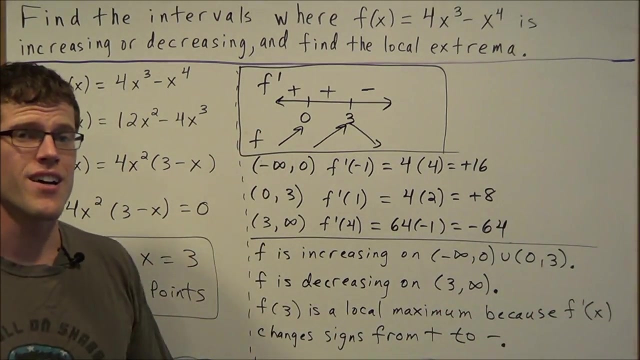 from positive to negative, which happens at x, equals 3.. So we can conclude that f of 3 is a local maximum, because the first derivative changes signs from positive to negative. Now just know, if we had to classify 0, we would say that f of 0 is neither a local.